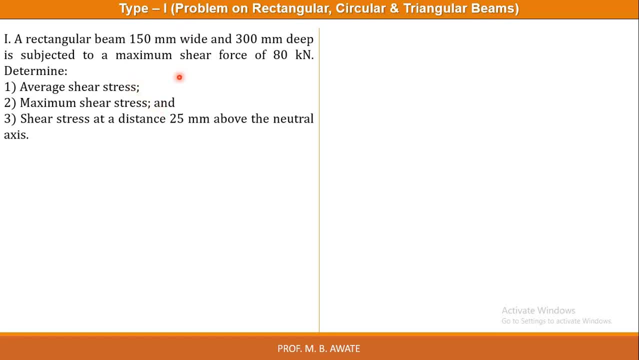 A rectangular beam 150 mm wide, 300 mm deep is subjected to a maximum shear force of 80 kN. Determine: average shear stress, maximum shear stress and the shear stress at a distance of 25 mm from the neutral axis. So the given data is: they have given the width B as 150 mm, depth D as 300 mm. 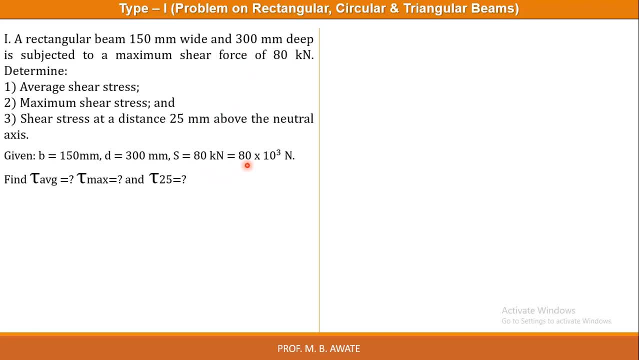 Also, the value of shear force is given as 80 kN. We are interested in finding out the value of average shear stress, maximum shear stress and also the shear stress at a distance of 25 mm from the neutral axis. So this is a figure. This is a rectangular section having breadth or width as 150 mm, depth as 300 mm. 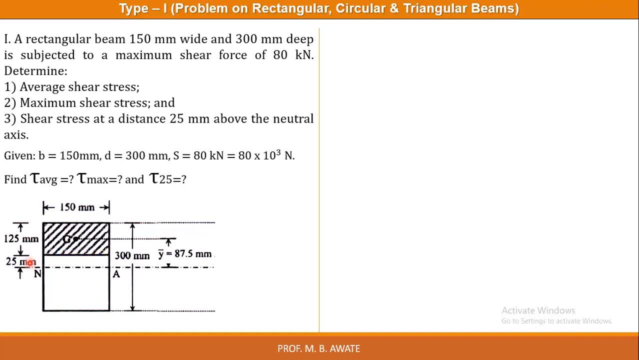 And this is a layer which is at a distance of 25 mm from the neutral axis And this particular shaded portion is nothing but the area above the neutral axis And, if at all, we want to find out the Cg of this particular area and its distance from the neutral axis. 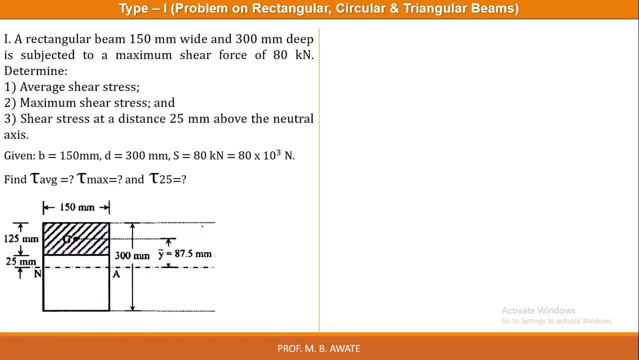 So it can be calculated like this, So that I will just extend like this here: So this total depth is half, Now total depth is 300.. So this distance is 150 mm, right, And here we know that this distance is 25.. 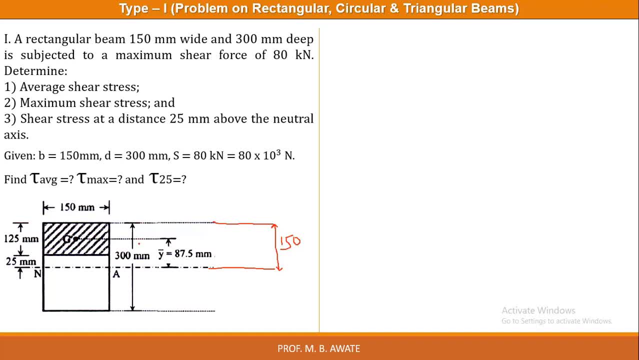 So remaining distance is also equal to 125.. And this half distance, I should say here, this half distance is what? 62.5 mm. Okay, This half distance is 62.5 mm And this 62.5.. 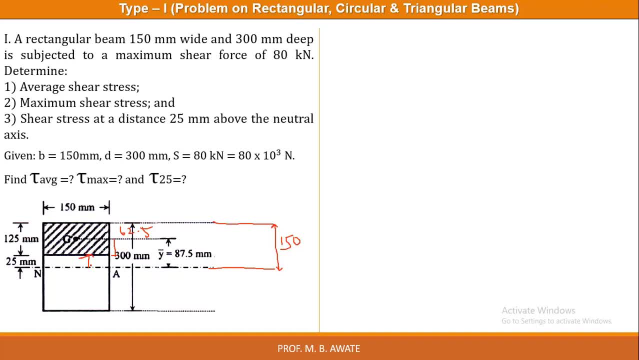 Plus this 25.. So that is nothing but this particular, This distance, 62.5, and this distance is 25.. Addition of both will give the value of y bar Means. distance of Cg of this particular area A from the neutral axis, which is equal to 87.5 mm. 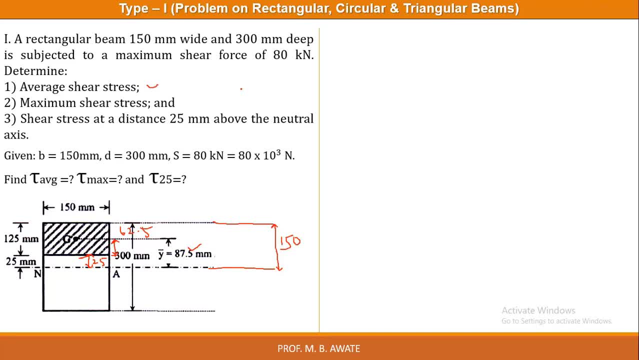 Now we will deal with our first objective. that is nothing but finding out the value of average shear stress. So average shear stress is given by tau. average is equal to 0.5.. So that is equal to S divided by A, where S stands for the shear force and A is nothing but area of a rectangle. 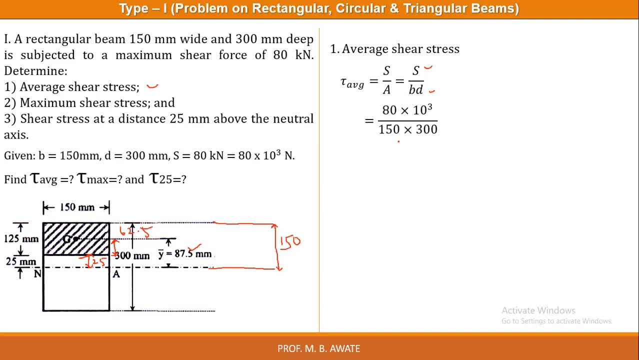 So S is equal to 80 into 10, raise to 3 and area is the product of B into D. Breadth of the rectangle is 150 and depth is 300. And from this I will get the value of average shear stress as 1.77 Newton per mm square. 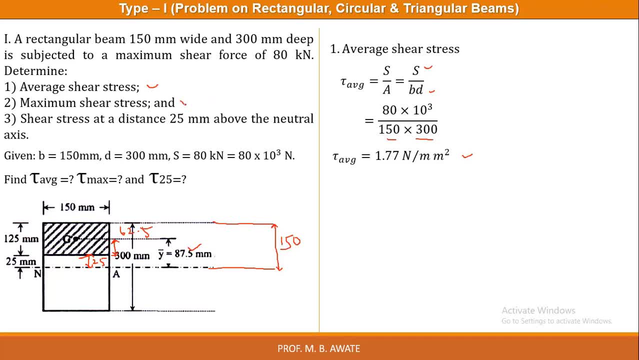 So we have done with our first objective. The second objective is to find out the value of maximum shear stress, And in the last lecture we have seen that the maximum shear stress occurs at the neutral axis as far as the rectangular section is concerned. 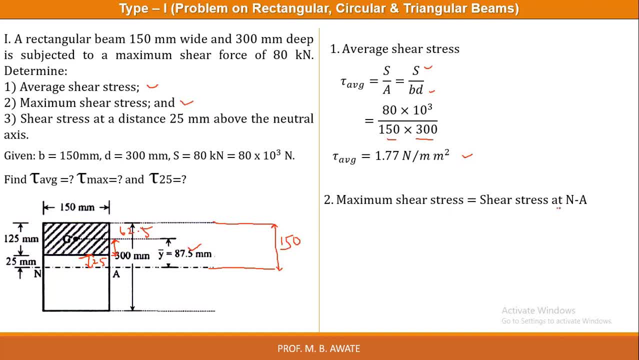 So maximum shear stress is nothing but the value of shear stress at the neutral axis And it is given by. maximum shear stress is equal to shear stress at the neutral axis. It is equal to 3 by 2 times average shear stress, or 1.5 times average shear stress. 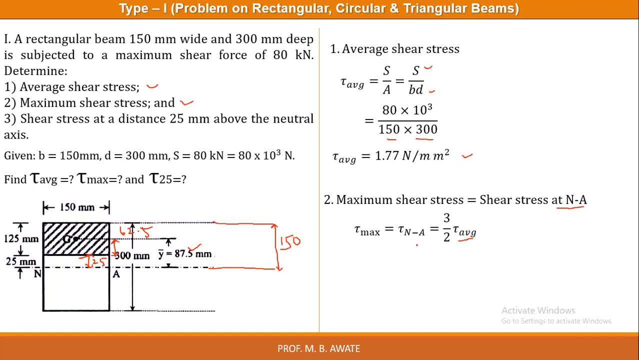 So already we have got the value of average shear stress here, which is 1.77.. So 3 by 2 into tau average and average shear stress is 1.77.. So we will be getting the value of maximum shear stress as 2.67 Newton per mm square. 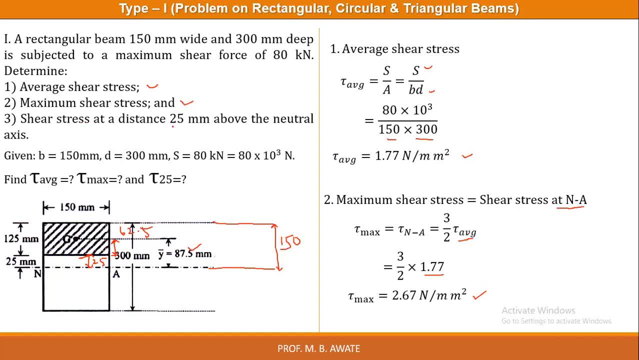 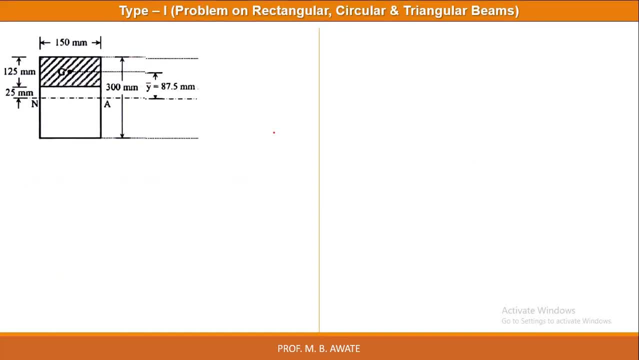 So we have done with our second objective. The third objective is to find out the shear stress at a distance of 25 mm above the neutral axis. So this will be the same figure. I am redrawing it, And this is the third objective. 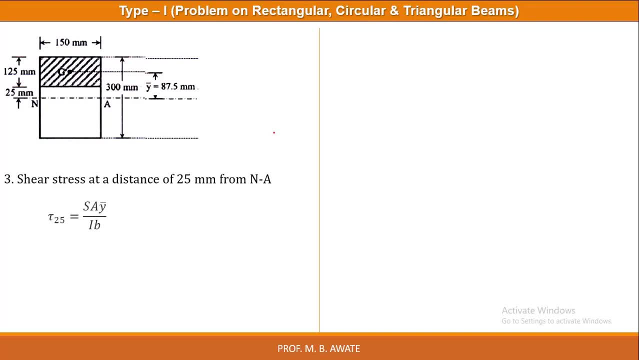 About finding out the shear stress at a distance of 25 mm above the neutral axis, And it is given by tau 25 means shear stress at a distance of 25 mm from the neutral axis is equal to S, a y bar upon i. So what are these elements? 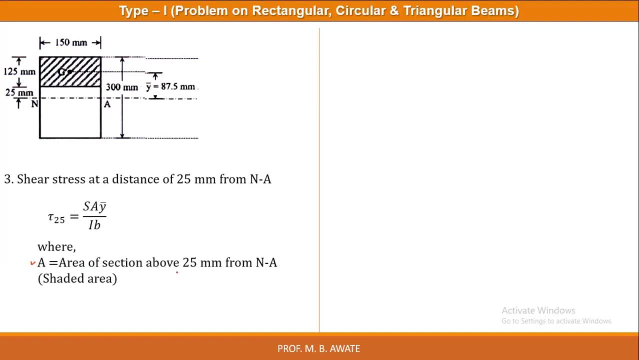 See here a. a is what Area of a section above 25 mm from the neutral axis. So this area which is shown by the shaded portion, This is area a y bar. So you can see here y bar. What is that? 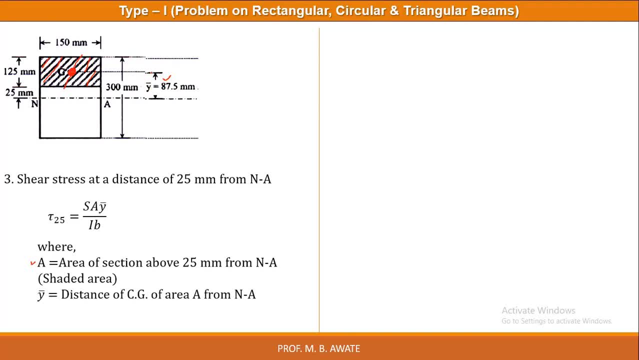 The distance of C, g of this particular area in this figure from the neutral axis. So the distance is y bar, which is equal to air 87.5 mm. This is y bar. i is sorry. b. b is what Width of the section at 25 mm from the neutral axis. 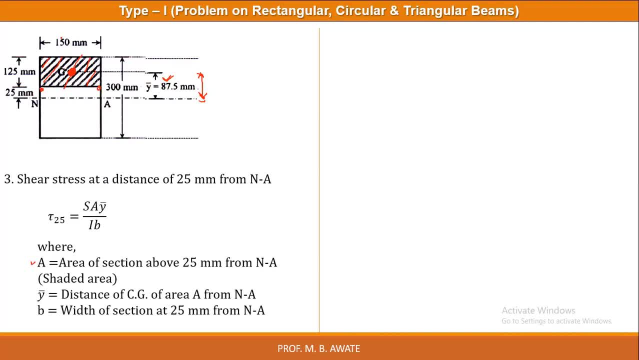 So if I will measure the width here also, So this width will be equal to 150 mm, because the cross section is uniform And i is nothing. but moment of inertia of this entire section means moment of inertia of this rectangular section about the neutral axis. 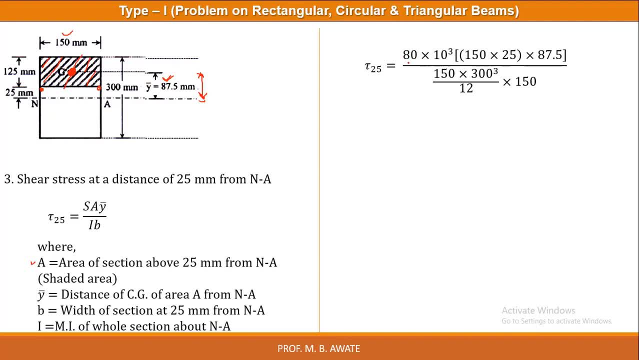 So tau 25 is equal to S a y bar upon i b. So this is the value of S shear force 80 into 10 raise to 3 Newton a is the area of a rectangle, which is 150 into 25, into y bar, which is equal to 87.5.. 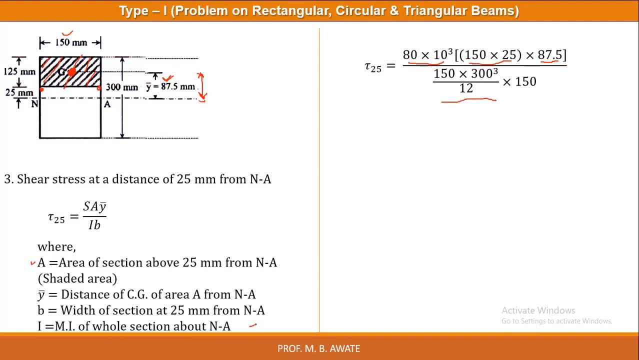 Divided by i. this is the moment of inertia of a rectangular section which can be given by the equation bd cubed by 12.. This we have seen in my last lecture. The moment of inertia for different cross section. It is bd cubed by 12.. 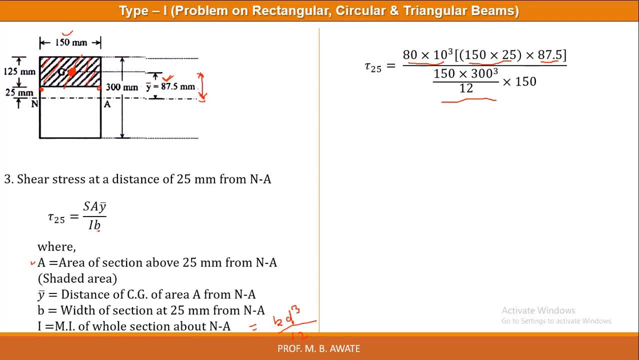 So b into d, cubed by 12.. This is moment of inertia. i and b. b is the width of the section, which is equal to 150 mm, And at the end I am going to find out, or I will be getting the value of. 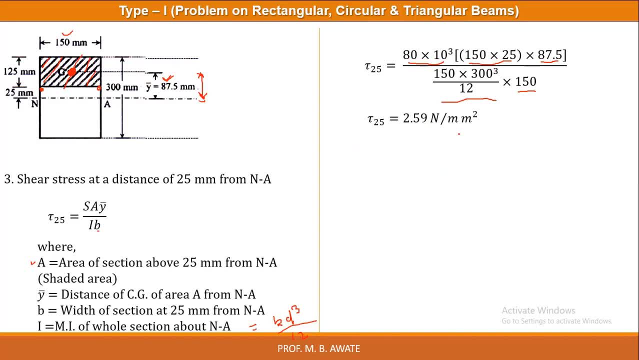 So the shear stress at a distance of 25 mm from the neutral axis is 2.59 Newton per mm square. This value I got for a layer at a distance of 25 mm from the neutral axis. Now we will plot the shear stress distribution diagram. 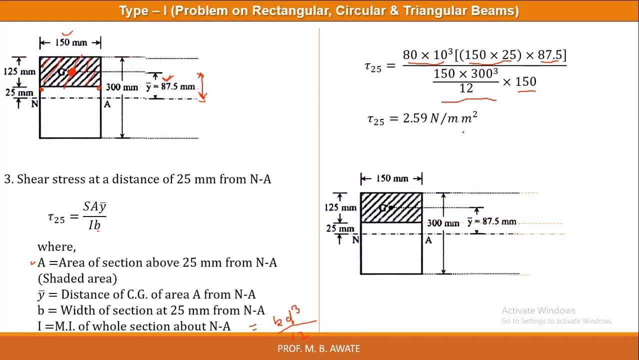 So this is the figure, And now we are just extending the lines, corresponding lines, And this is the vertical line And from this I am going to mark the values. So at this point I will say This is the at the neutral axis. 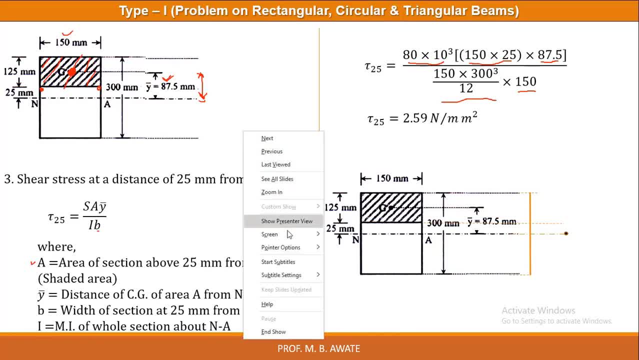 And here the shear stress will be. I will say, At this particular point The shear stress will be maximum, Which is equal to Here, 2.67 Newton per mm. square. The next point Is the shear stress at a distance of 25 mm. 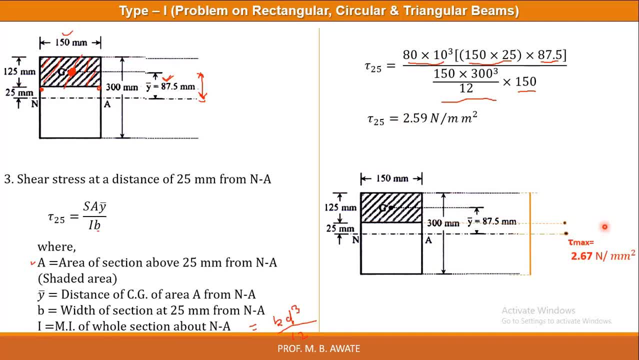 Where the value is 2.59.. So it is just behind this Shear stress at a distance of 25 mm From the neutral axis, And that is. value is 2.59 Newton per mm square. Now We will draw the shear stress distribution diagram. 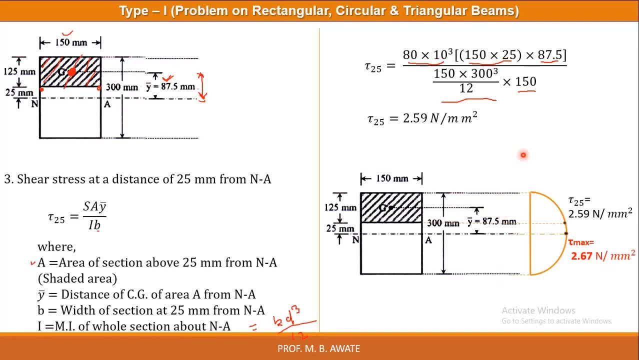 For this rectangular section And it will be like this. So this is nothing but The problem on A rectangular beam And we have done Or we have calculated The values of shear stresses At the neutral axis And also at a given distance. 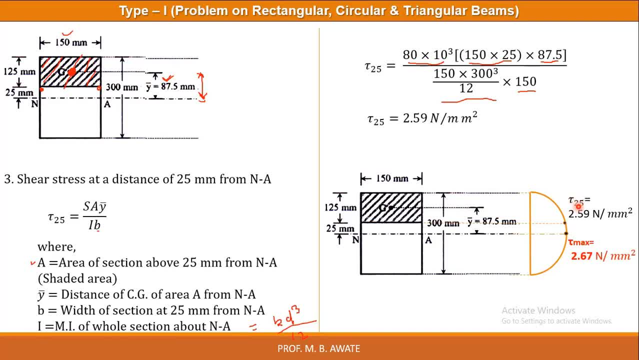 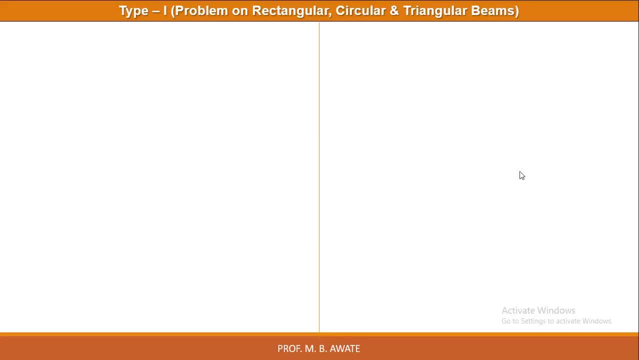 From the neutral axis. That is nothing but Shear stress at a distance of 25 mm From the neutral axis, And for that We have drawn the shear stress distribution. Now We will see the next problem. So the problem statement is: 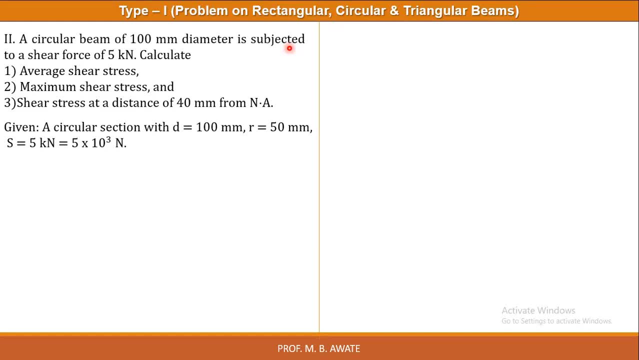 A circular beam Of 100 mm diameter Is subjected to a shear force of 5 kN. Calculate Average shear stress, Maximum shear stress At a distance of 40 mm From the neutral axis. So this is the problem statement. 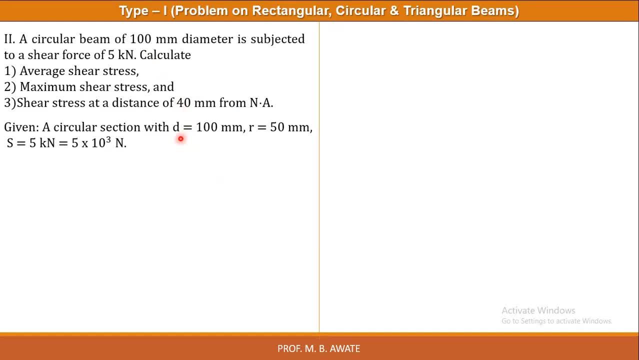 And from that We can write down the given data like this: Diameter is 100 mm. Radius r is equal to 50 mm. The shear force carries the value of 5 kN, Or 5 into 10 to 3 N. 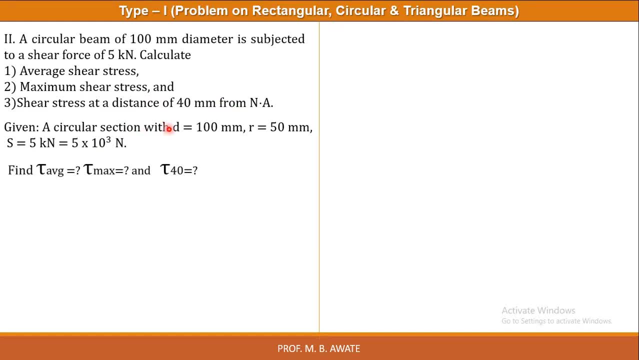 And We will draw the figure for the same. These are the objectives: Tau average, Tau max And Tau at a distance of 40 mm, Which is a section, Circular section of a beam Which is having a diameter 100 mm. 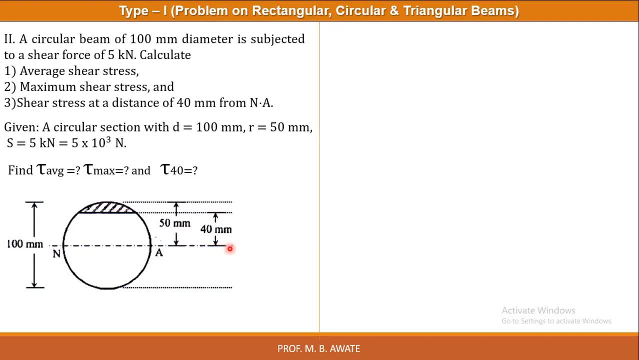 Radius 50 mm, And here we have shown a layer Which is a distance of 40 mm from the neutral axis. So we will deal with our first objective, That is, to find out the value of Average shear stress. The average shear stress. 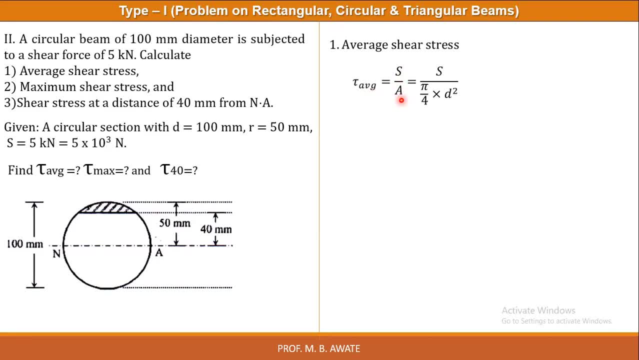 Is given by Tau. average is equal to s divided by a, And a is nothing but pi by 4 into d square. As it is a circular section And the value of shear force s Is 5 into 10, raise to 3.. 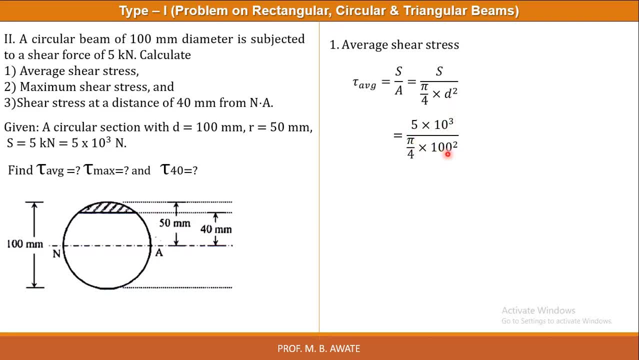 And the diameter is 100 mm. So pi by 4 into 100 square. So I am going to get The value for average shear stress as 0.066366 N Per mm square. So this is the average shear stress. 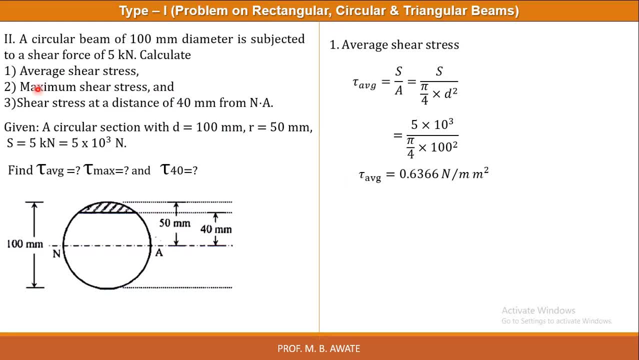 In a rectangular section. Now we will deal with our second objective, That is, to find out the maximum shear stress, And we know that for a circular section Maximum shear stress always Occurs at the neutral axis. That we have seen In that last lecture. 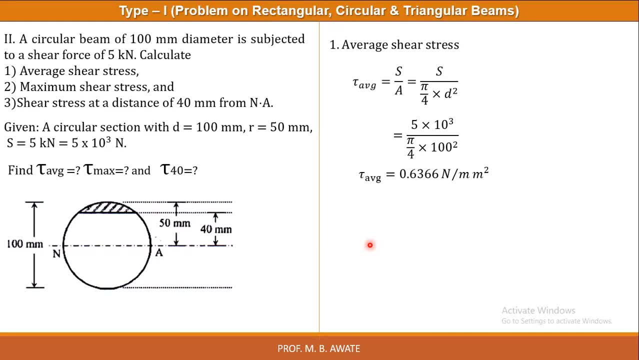 So if at all you want to just revise it, Go through that last lecture Where I have explained The shear stresses and their distribution In various cross sections. So now the maximum shear stress In a circular section. It occurs at the. 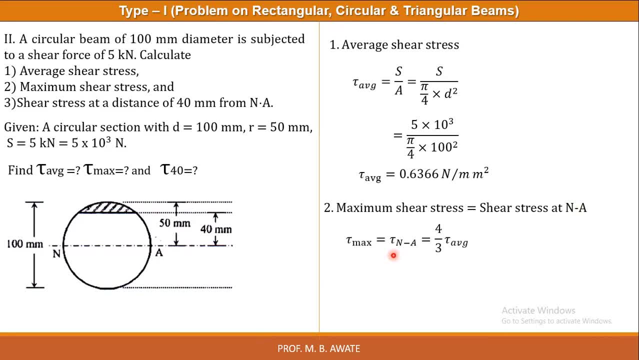 Neutral axis And tau max is equal to Tau at the neutral axis. That is nothing but 4 by 3 times tau average. This equation also we have seen In my last lectures. So tau average we are knowing The value is 0.6366.. 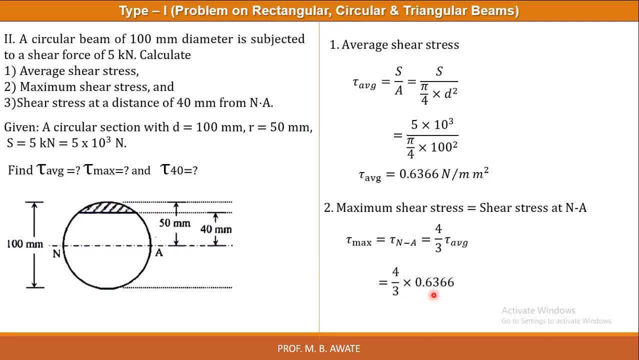 So just replace Tau average by that value, 4 by 3 into 0.6366.. So at the end I am going to get the value of tau max as 0.8488 N Per mm square. So this is the value of maximum shear stress. 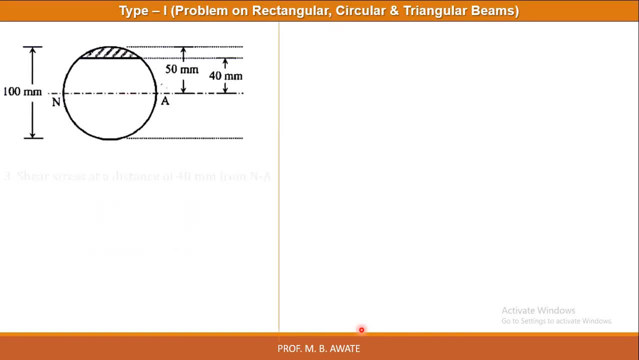 Which is acting at the neutral axis. Now the next point is: We have to find out the shear stress At a distance of 40 mm from the neutral axis, And it is given by The equation Tau, 40 means shear stress. 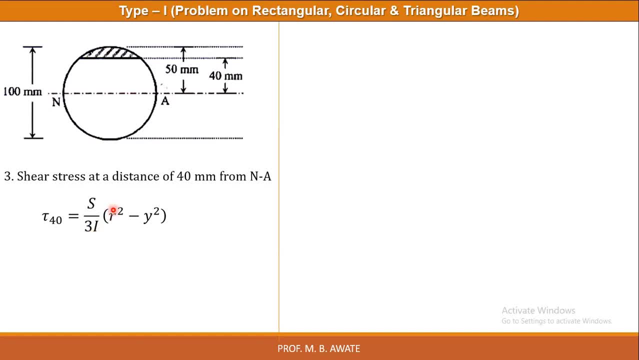 At a distance of 40 mm from the neutral axis Is equal to s divided by 3i Into bracket r square minus y square. This equation also I have already explained in my last lectures. You just go through those lectures Where I have explained the shear stresses. 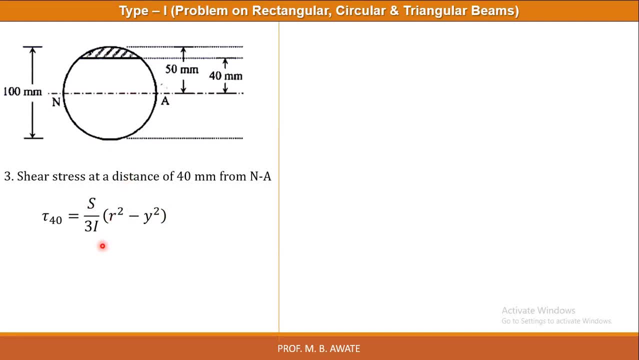 Across various cross sections. So s is the shear force. i is the moment of inertia of a circular section. r is the radius Of a layer, So we will just keep these values. So i is nothing but Moment of inertia of a circular section. 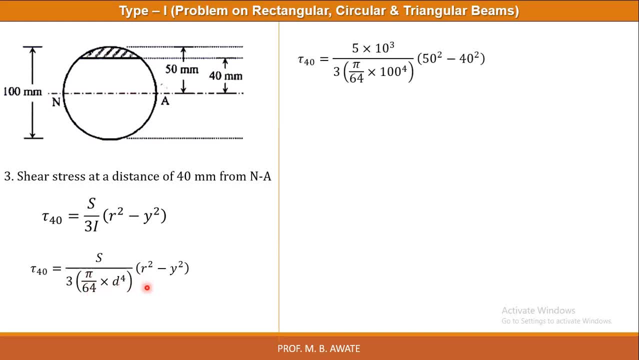 Which is given by pi by 64 into d raise to 4.. And I am going to replace all these values Like s is 5 into 10 raise to 3.. i 3 times, i means 3. Into pi by 64 into d raise to 4.. 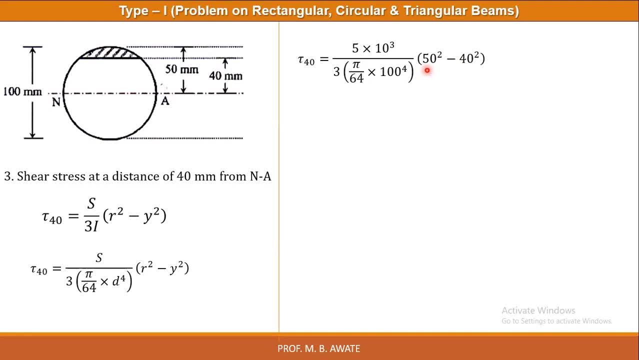 Where d is 100 mm Into r square minus y square, So r radius is 50.. 50 square minus y Distance is 40 mm from the neutral axis, So from that I will be getting The value of shear stress at a distance of. 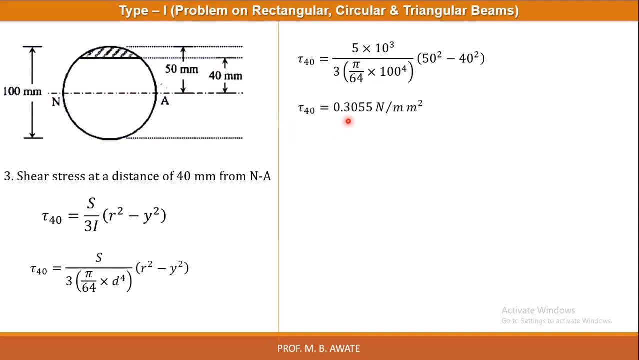 40 mm from the neutral axis as 0.3055 Newton per mm square. So this is the value of a Shear stress at a distance of 40 mm from the neutral axis. Now the next thing is We have to plot the shear stress distribution. 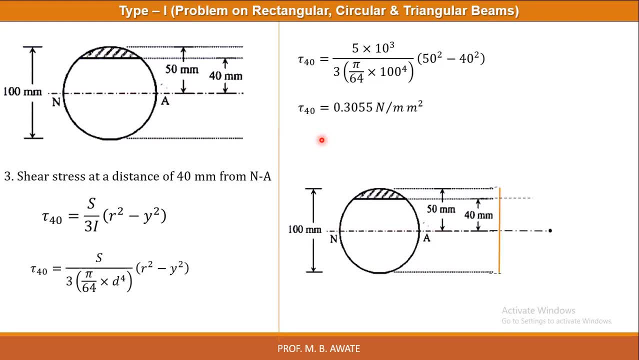 Diagram. So the maximum shear stress: here You can see it is occurring Or it is at the neutral axis, Which is having a value of 1.33 Newton per mm square. Now, here, at this point, I will mark the value of a shear stress. 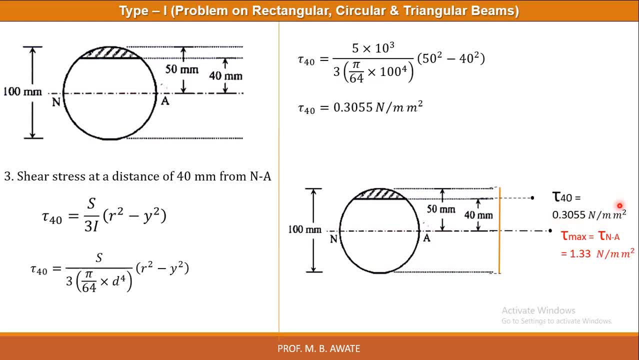 At a distance of 40 mm. That is equal to 0.3055 Newton per mm square, And I will draw The distribution Shear stress distribution curve. So this is nothing but The problem on circular section. Now we will move on. 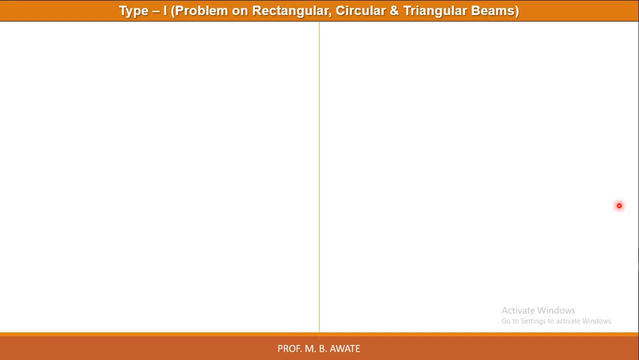 To our next problem. That is nothing but the problem on Triangular section. I will read the problem. The scheme of triangular section Has a base 90 mm And a height 120 mm If the section Is subjected to a shear force. 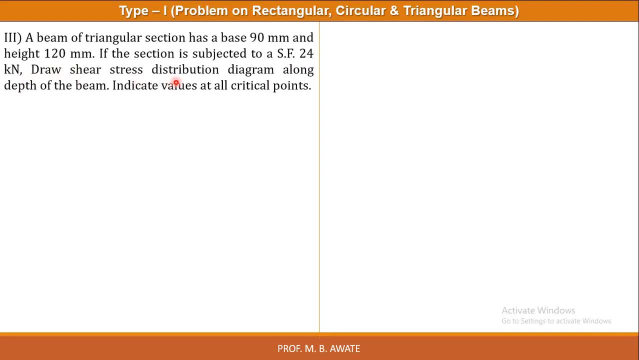 24 kilo Newton. Draw the shear stress Distribution diagram Along the depth of the beam And indicate values At all the critical points. So here We are knowing the dimensions of the triangle And value of shear force. I will write as a given content. 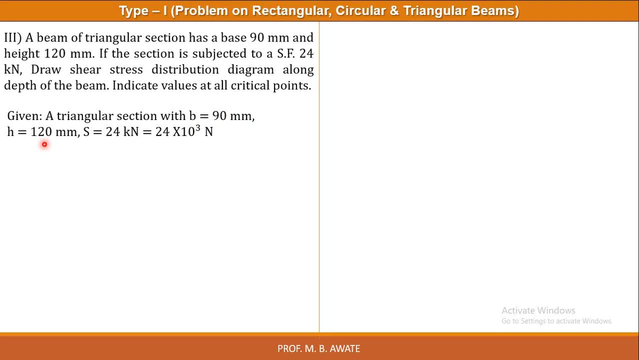 So base 90 mm, Height as 120 mm And shear force as 24 kilo Newton, That is nothing but 24 into 10 to the power 3 Newton And we have to find out the shear stress At the neutral axis. 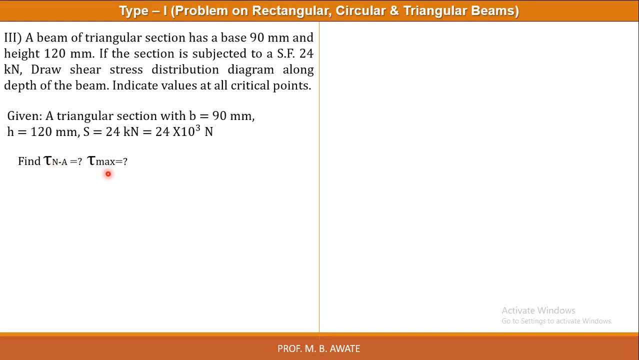 That is nothing but Sorry. we have to find out the shear stress at the neutral axis And also we have to find out the maximum shear stress For a triangular section, And this is the figure In this figure That This is a triangle having base 90 mm. 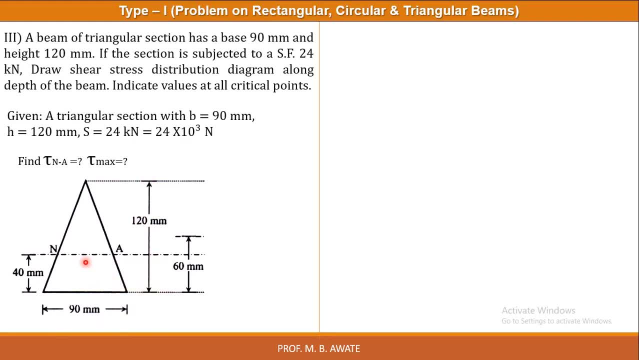 Height as 120 mm And we know that The shear stress, Sorry, the CG- is At a distance of CG, you can see, Is at a distance of 40 mm, Because height is 120 mm And CG occurs. 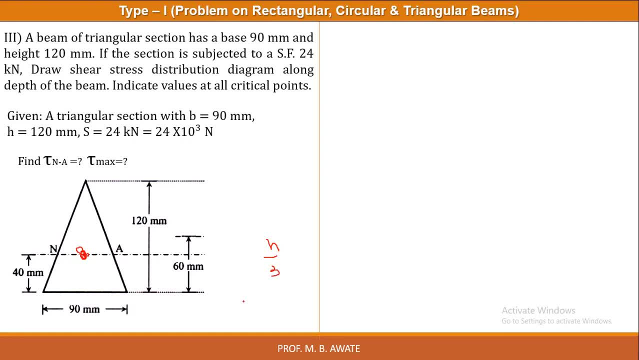 At a distance of h by 3. From the base, So height is 120.. And divide by 3., So that is equal to 40. So that we have shown here Distance as a 40 mm. And I have also taken the half distance. 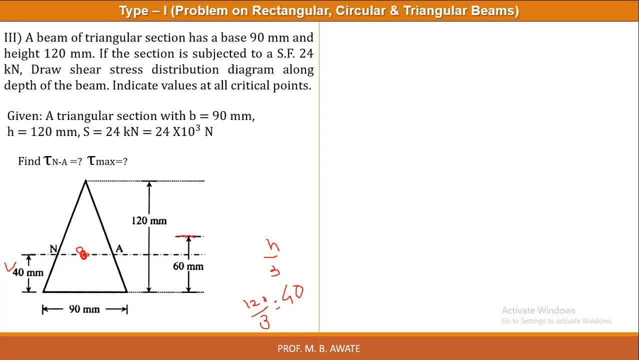 60 mm. The total height is 120.. I have taken the value as a 60 mm Because for a triangular section The maximum shear stress occurs At a half of the distance of height. So here there will be the maximum shear stress. 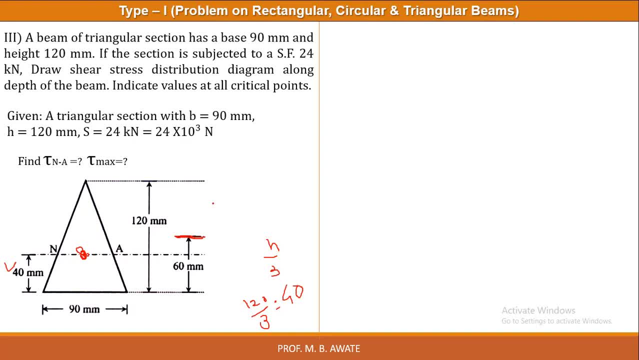 Which is acting In this triangular section. So initially we have marked The significant points. Now we will try to find out the value. Now we will find out the average shear stress In this particular triangular section, And average shear stress Is given by: 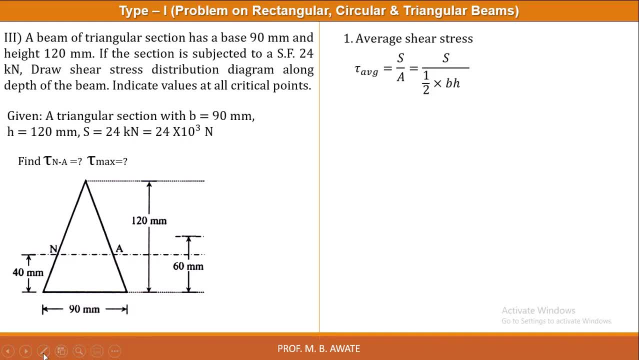 S divided by A, Where S is the value of a shear force And A is nothing but The area of the triangle. So S square is the value of 24 kilo Newton. 24 into 10 raise to 3.. 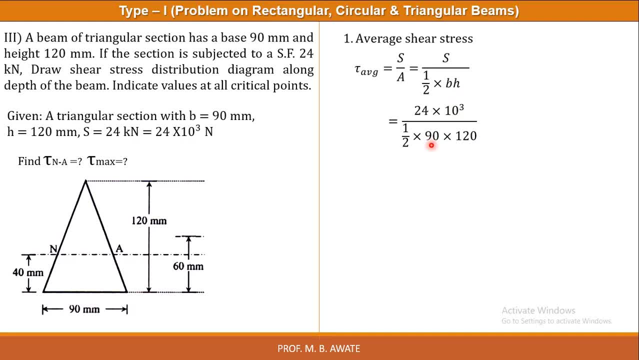 And area is 1 by 2 into base, into height, So 1 by 2 into 90, into 120.. So I will be getting the value of Average shear stress as 4.444 Newton per mm. Now, As we have calculated, 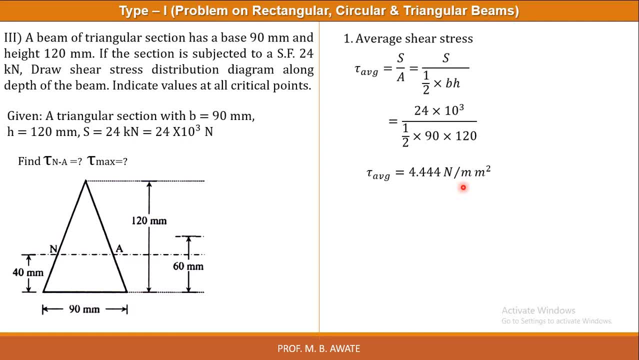 The average shear stress. The next thing is that I will calculate the shear stress At the neutral axis, And we know that the neutral axis Is lying at a distance of 40 mm From the base. So Shear stress at the neutral axis. 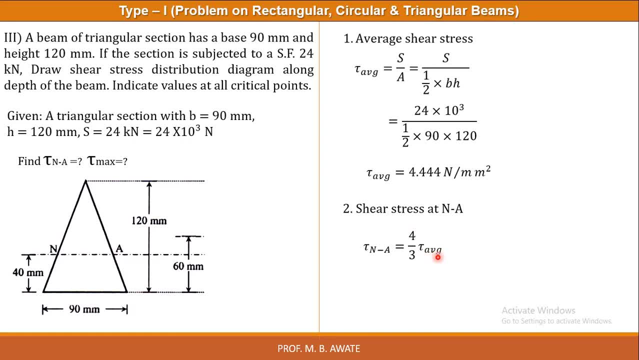 Is 4 by 3 times The tau average, 4 by 3 times the average shear stress, So 4 by 3.. Into 4.444.. So average shear stress, Or multiplied by 4 by 3.. 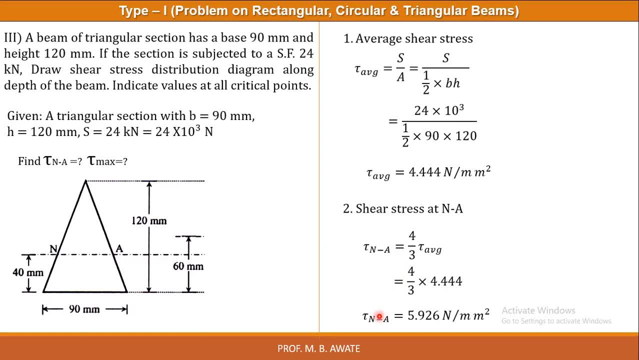 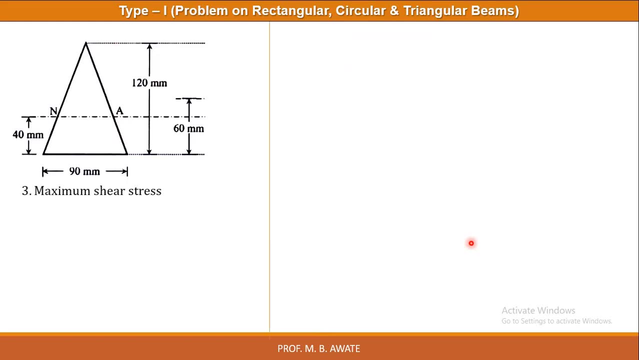 I am going to get the value of Shear stress at the neutral axis As 5.926 Newton per mm square. So this equation We have already seen for the triangular section In my initial lectures. Okay, Now What is the value of a maximum shear stress? 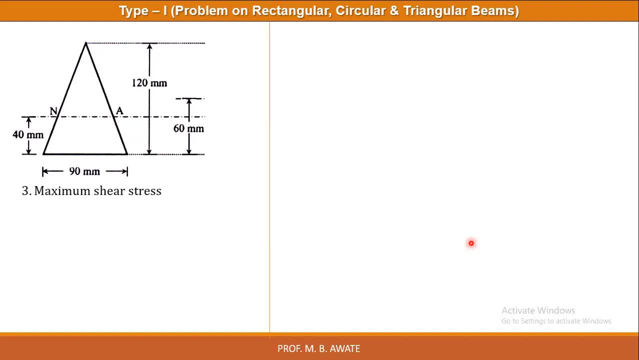 And for a triangular section, The maximum shear stress always occurs. Always occurs at a Half of the distance of its height Means. it is occurring at a distance of 60 mm And generally It is given by the equation. Maximum shear stress is given by the equation. 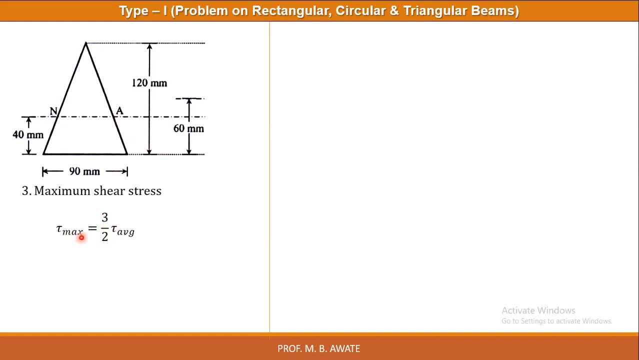 Tau max is equal to 3 by 2 times tau average, Or tau max is equal to 1.5 times tau average. This relation also I have explained in my last lectures. So Tau max is equal to 3 by 2 into 4.44.. 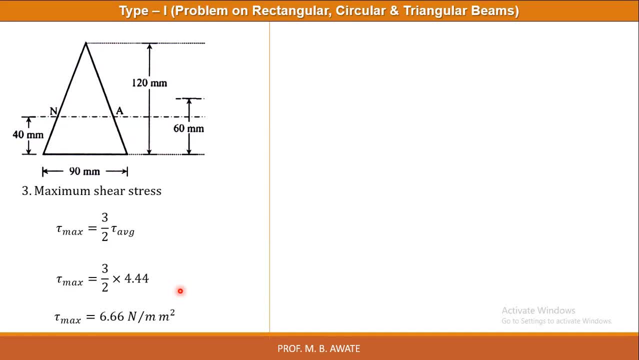 So maximum shear stress is equal to 6.66.. Newton per mm square. So this is the value of Maximum shear stress, And maximum shear stress occurs At a distance of h by 2. From the base For a triangular section. 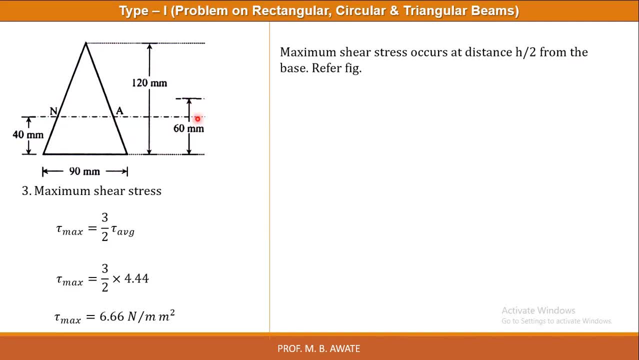 So refer figure Okay, Distance is 60 mm, Or I will say Half of its height. If you measure from the top As well as from the bottom, Distance is going to remain same, Which is equal to 60 mm. 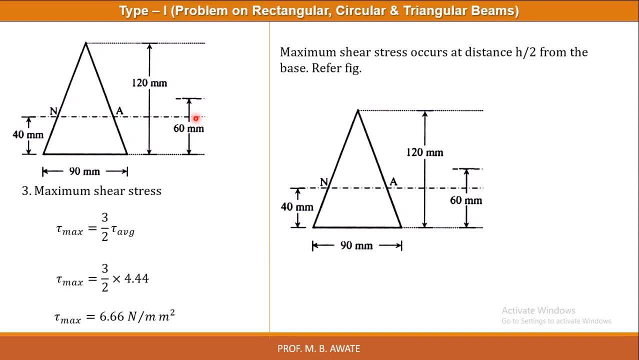 Now We are interested in finding out, Or we are interested in drawing The shear stress distribution diagram As far as This particular triangular section is concerned. Okay, So we will just extend the lines. So this is line Extending from the top surface. 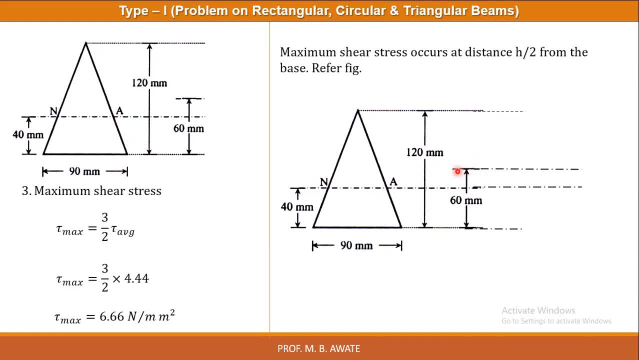 This line is from the Height h by 2. Of this particular triangle And this is the line From the neutral axis. Now We have taken One reference line And we have marked the first point At a distance of 60 mm. 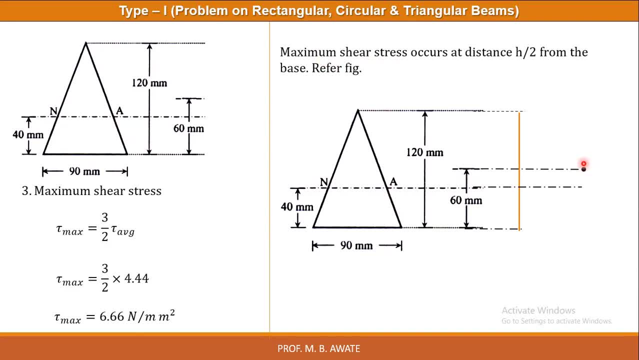 And here you can see, The shear stress will be maximum, Which is equal to Tau. max is equal to 6.66.. Newton per mm square. And now we are marking the shear stress At the neutral axis, Which is having the value of